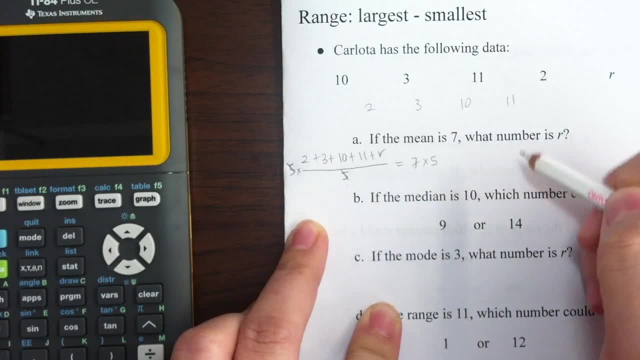 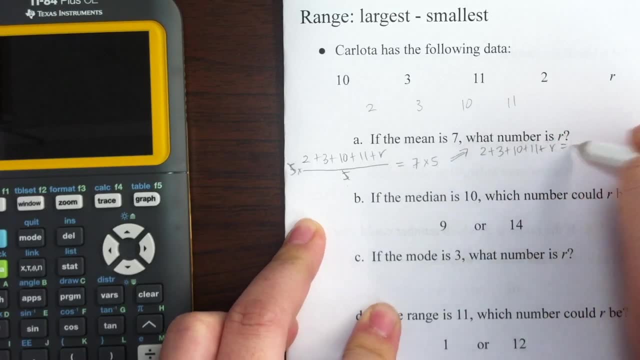 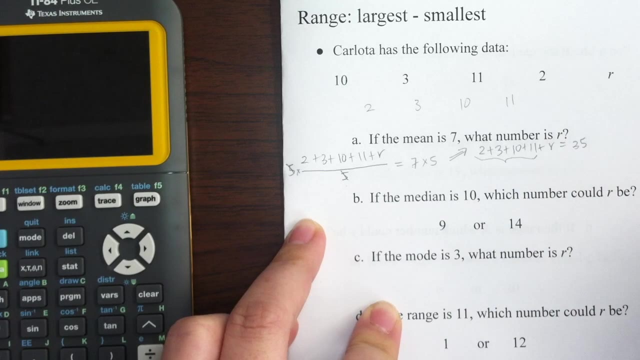 5 divided by 5 is 1.. 7 times 5 will be 35. So 2 plus 3 plus 10 plus 11 plus R equals 35. Now I can simplify: 2 plus 3 plus 10 plus 11.. 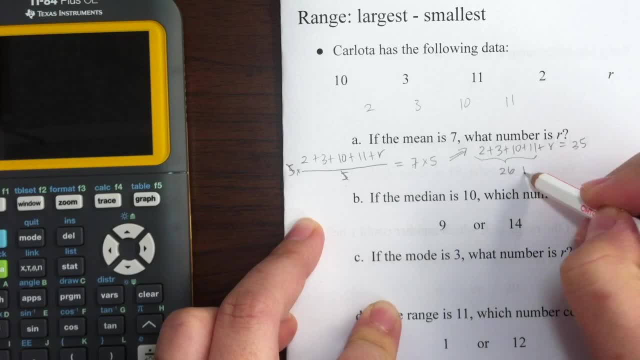 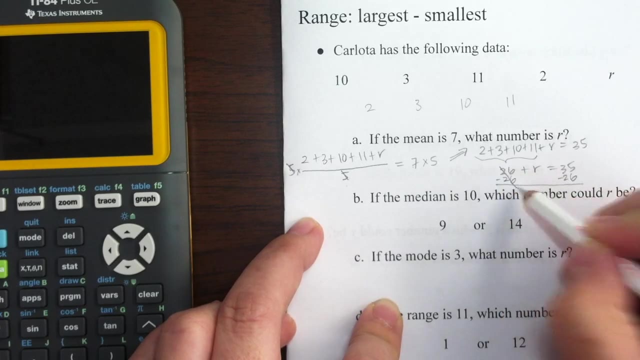 And that will give me 26.. Now I have 26 plus R equals 35. Here I have a sum, so I change the sign to minus Minus 26 on both sides. 26 minus 26 will eliminate And R equals 35 minus 26,, which is R equal to 9.. 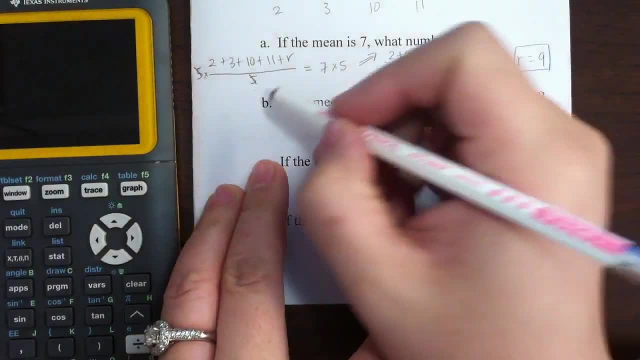 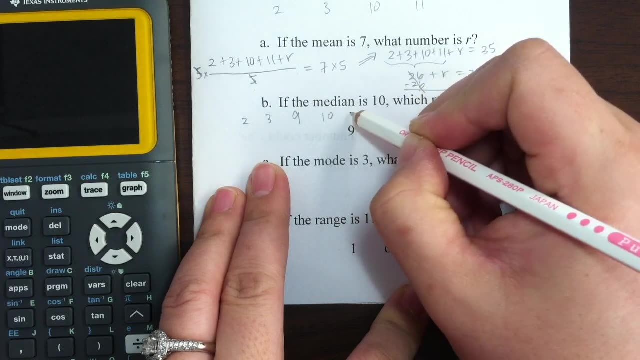 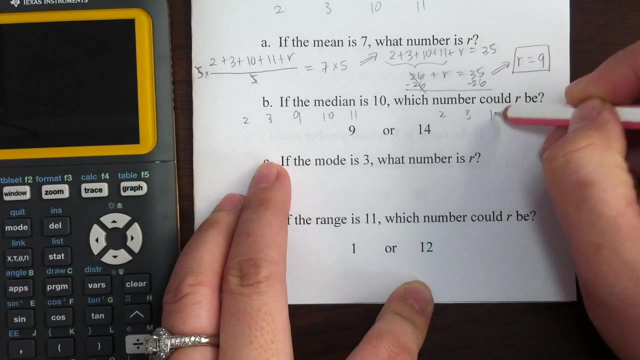 If the median is 10, what number could R be? I'm going to rewrite the numbers with 9 this time And then separately rewrite the numbers with 14.. 1,, 2,, 3,, 10,, 11,, 14.. 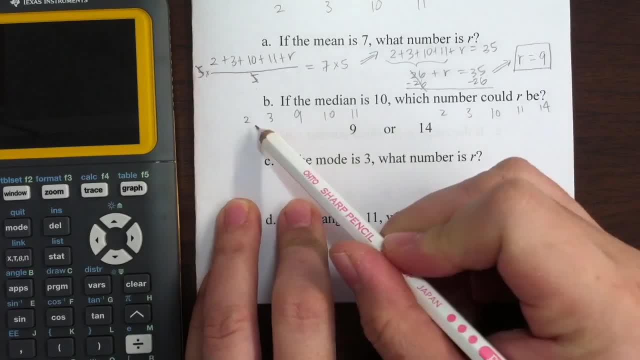 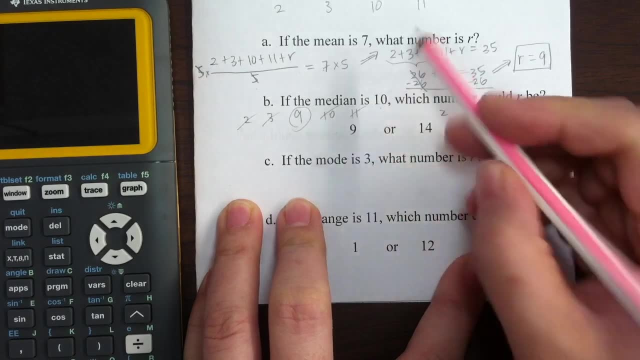 So I check here: What is the median? I eliminate the outside numbers, The middle is 9.. But I want the median to be 10.. So it's not 9.. Over here: I eliminate the outside numbers, My median is 10.. 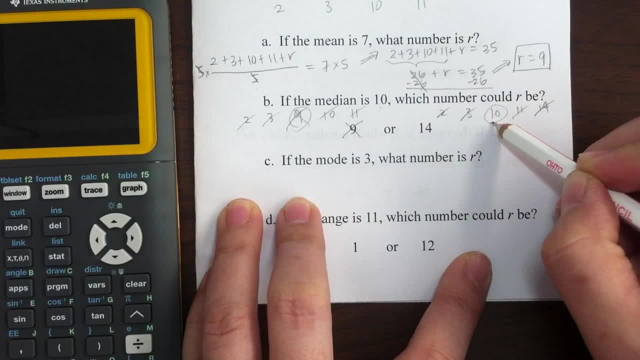 So my answer R should be 14.. If the mode is 3,, what number is R? Remember mode is the most important number. So, if the number is 3,, what number is R? Remember mode is the most important number. 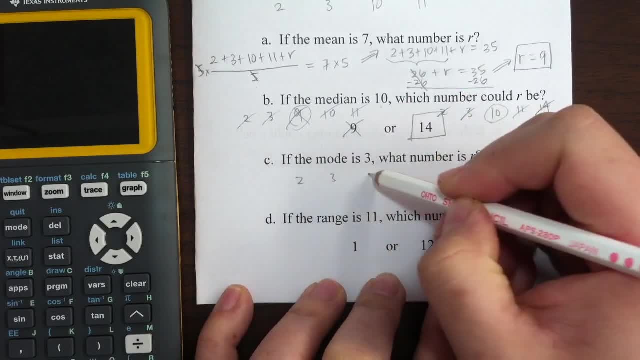 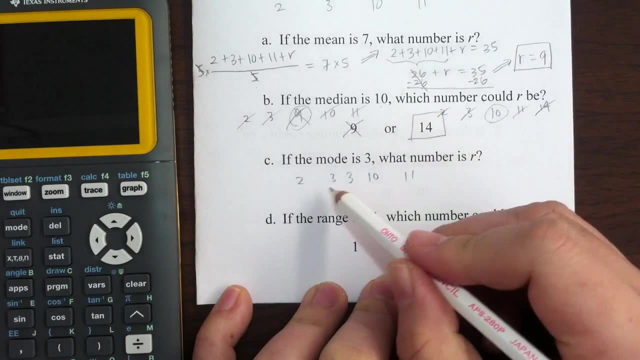 So if the number is 3, what number is R? Remember mode is the most important number If the number is the most common. right now there is no repeated number, So I need to repeat the 3 to make it the most common. So R equals 3.. If the range is 11,, which number should R be For the range? If I add in 1,, the range is the largest number minus the smallest number, 11 minus 1, which is 10.. 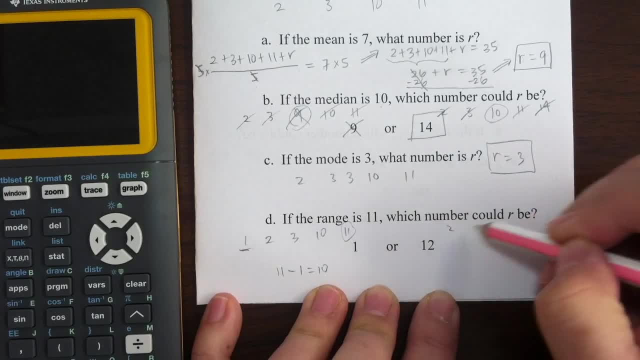 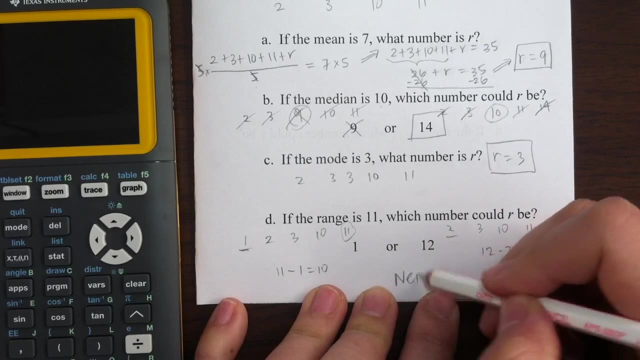 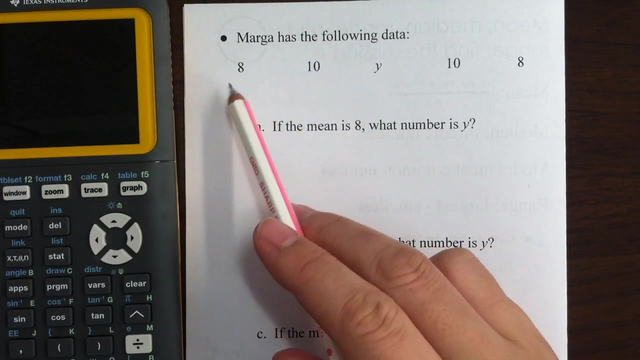 11 minus 1,, which is 10.. in 12,, then it's the largest minus the smallest, 12 minus 2,. 12 minus 2 equals 10, so in this case it's neither. Marga has the following data: 8,, 10,, y, 10, and 8.. 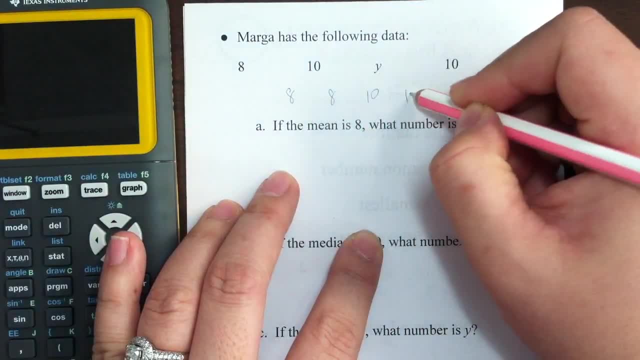 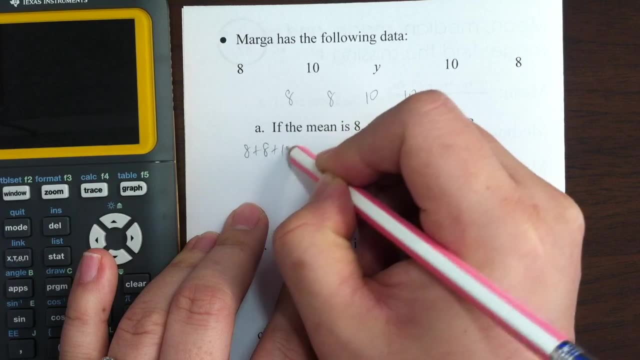 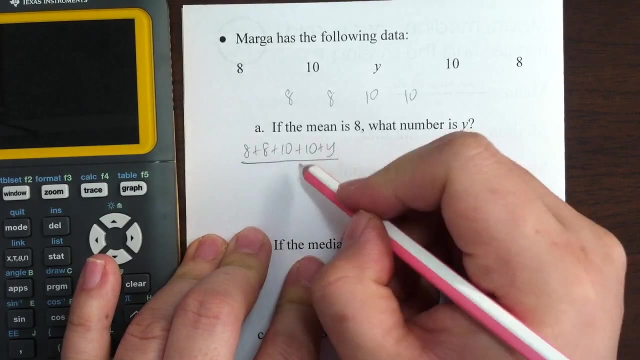 Again. I'm going to write these in order just to make it a little easier for myself. I want the mean to be 8, and I need to find y. So 8 plus 8 plus 10 plus 10 plus y over 1,, 2,, 3,, 4, 5 numbers equals mean of 8.. 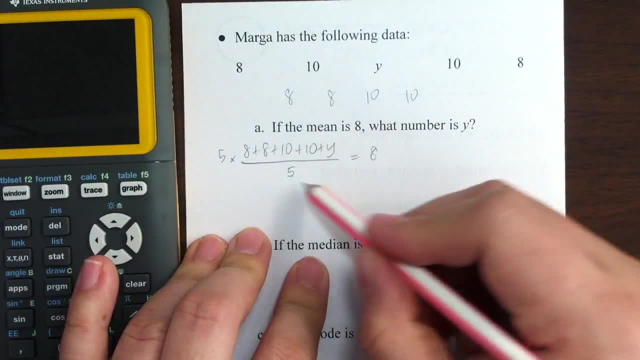 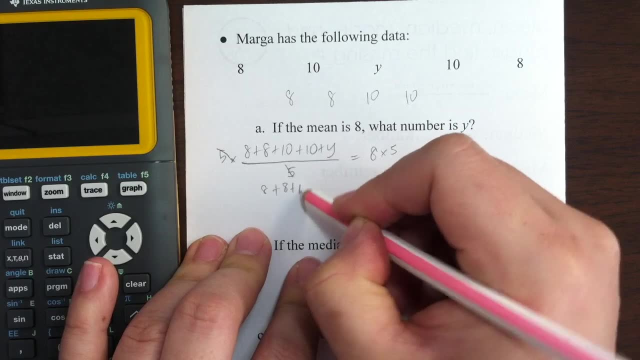 Again, I need to eliminate the 5, so I multiply, because that's the inverse of division: 5 divided by 5.. So 8 is 1,, 8 plus 8 plus 10 plus 10 plus y equals 40.. 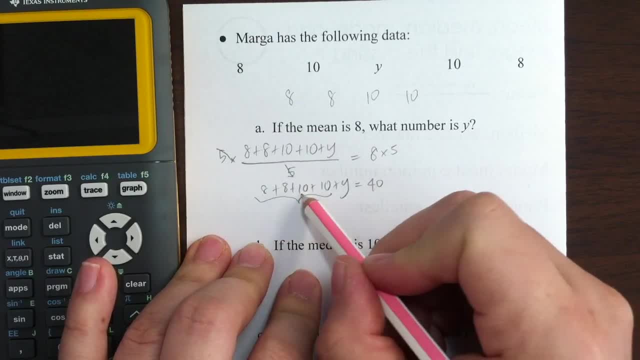 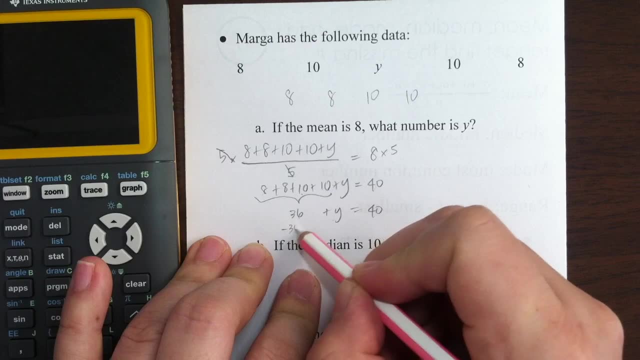 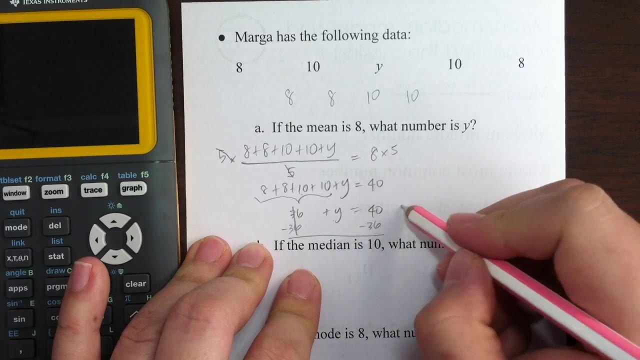 And I can simplify: 8 plus 8 plus 10 plus 10 is 36, and then I subtract 36 from both sides to eliminate the 36, and I have y equals 40 minus 36.. So y equals 4.. 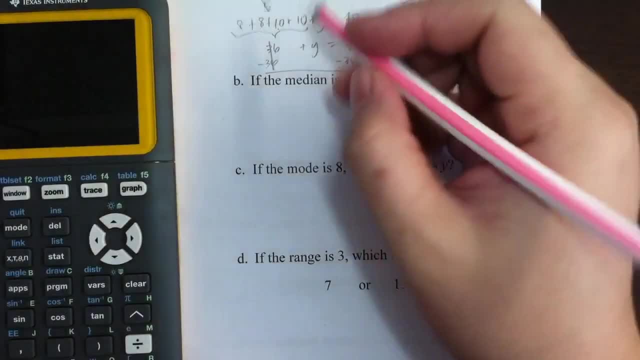 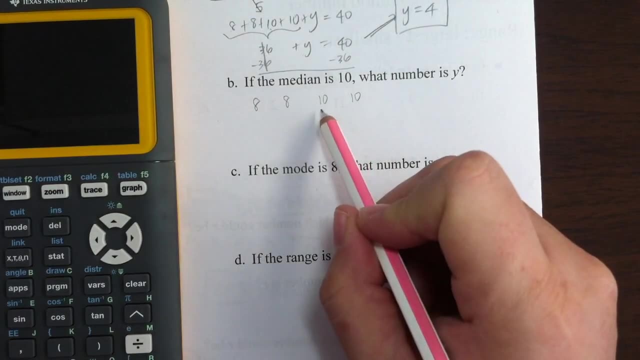 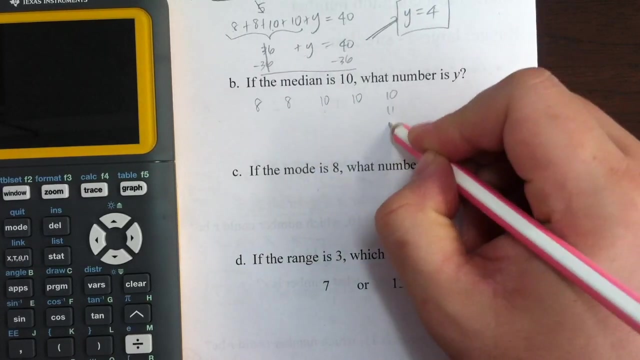 If the median is 10, what number is y? I'm going to rewrite the numbers. I want 10 for the median. I want it in the middle, So y can be 10,, it can be 11,, 12, or any number that's bigger than 10.. 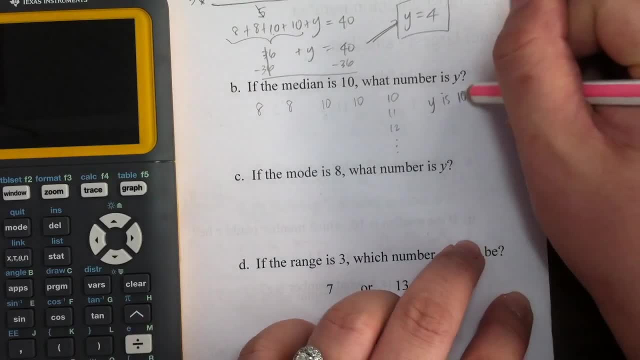 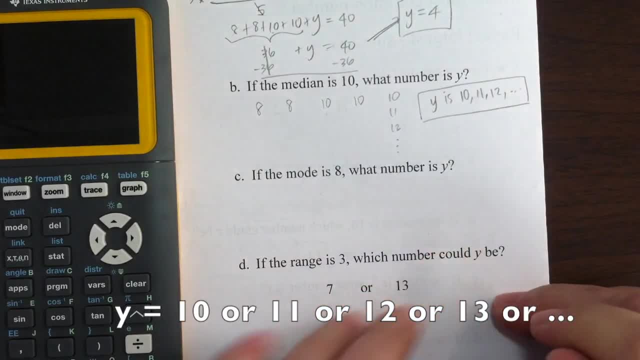 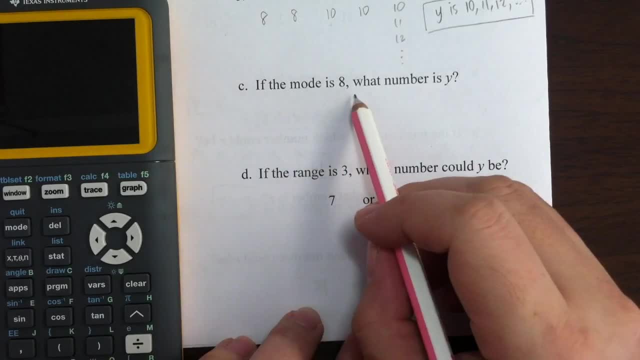 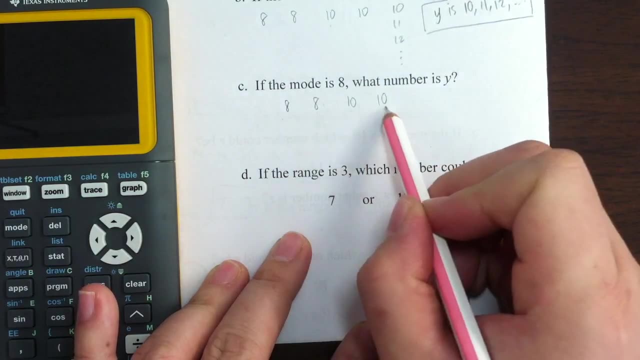 So y is 10, or 11, or 11, or 12, or 12.. So y can be any number, 10 or larger. If the mode is 8,, what number is y? Currently I have 8 repeated and 10 repeated. 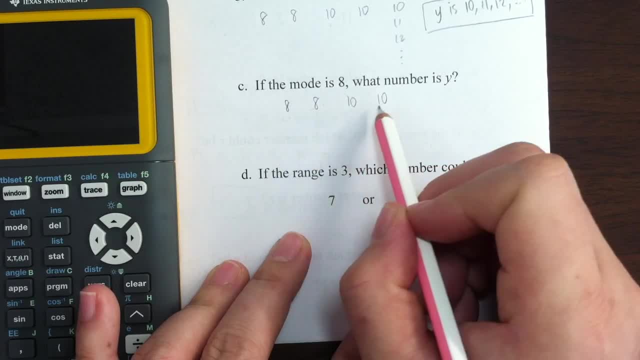 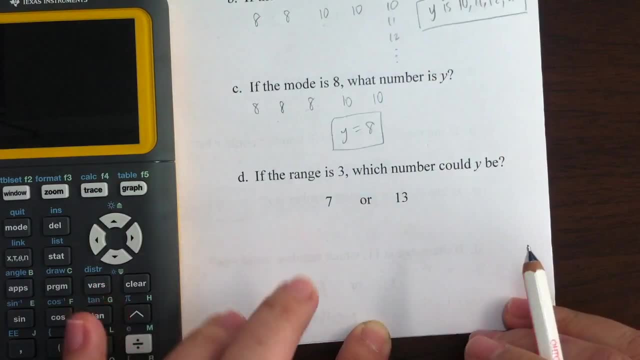 But I want the mode to be 8, so I need 8 to be more common than 10.. I need it to be repeated more times, So it must be 8.. y equals 8.. Finally, if the range is 3, what number could y be? 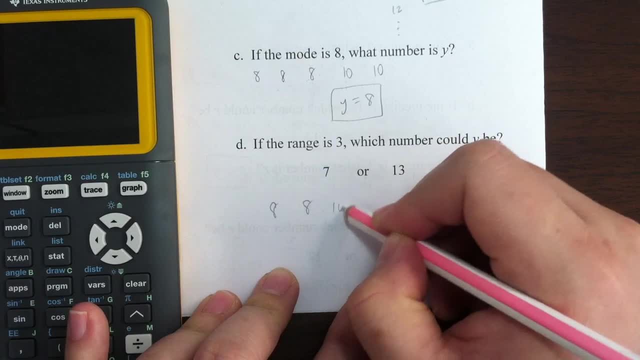 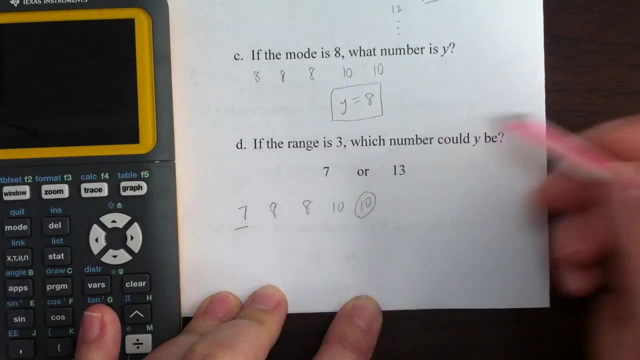 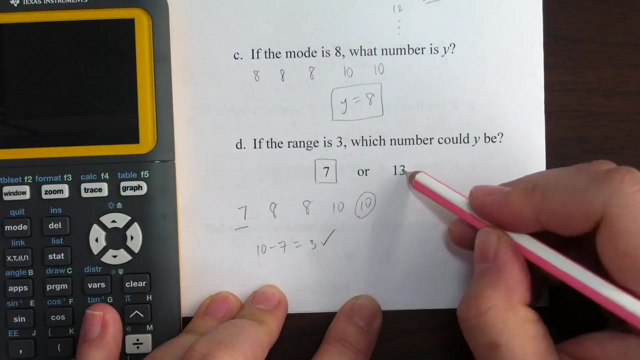 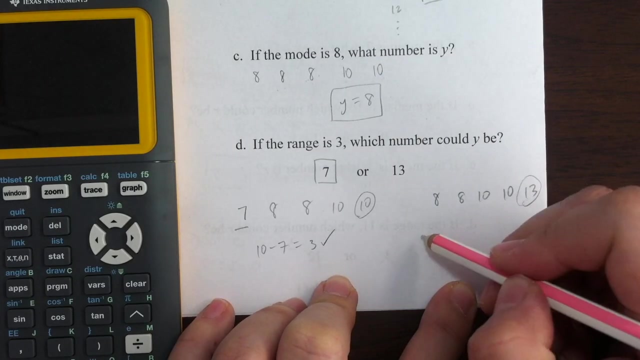 y equals 3.. YB: If I put 7 in here, then the range is the largest number minus the smallest number, 3, which is what I want. Just to check, I'm going to use 13.. So the largest number 13,. 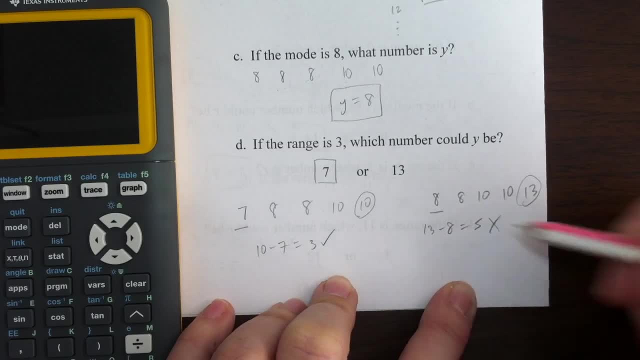 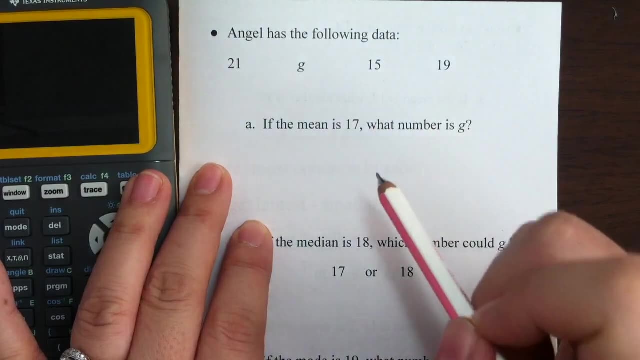 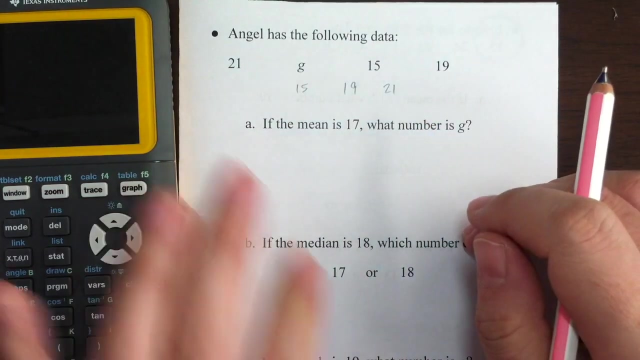 minus the smallest number, 8,, is 5,, not what I want. Angel has the following data: 21,, G, 15, and 19.. I'm going to write these in order again, And I don't know where G goes. 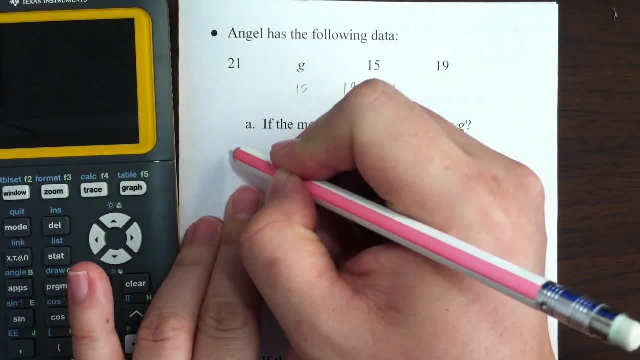 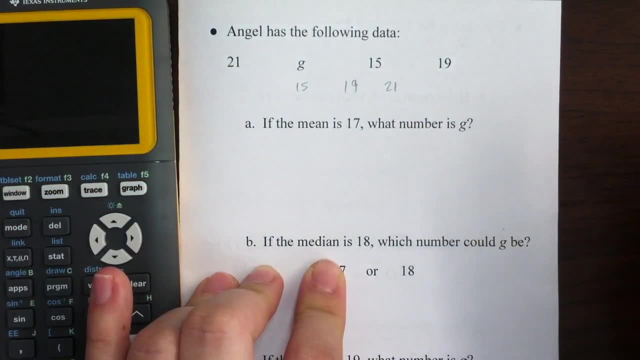 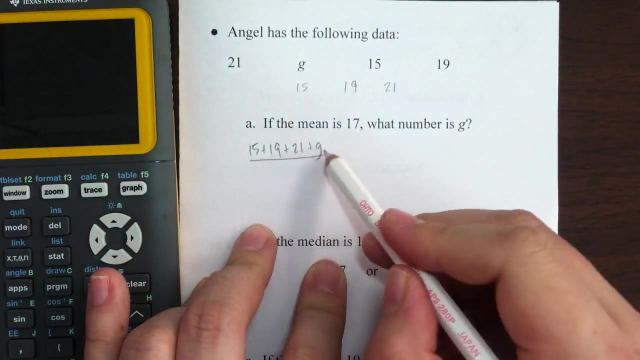 If the mean is 17,. what number is G? So 20.. So So 15 plus 19 plus 21 plus G, divide 1,, 2,, 3, 4, equals 17.. I need to eliminate the 4.. 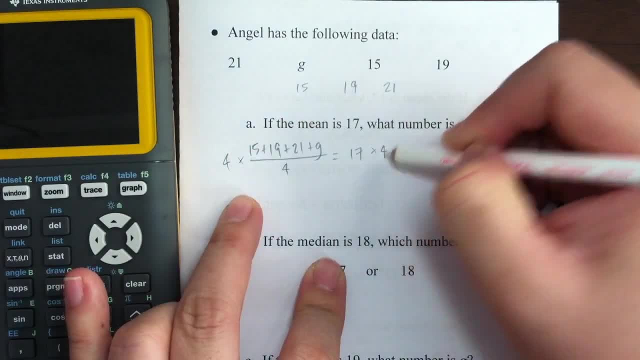 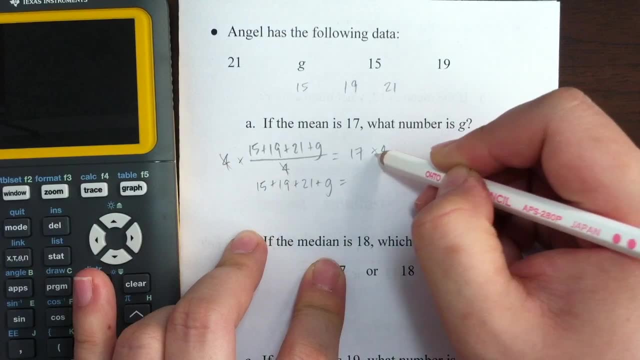 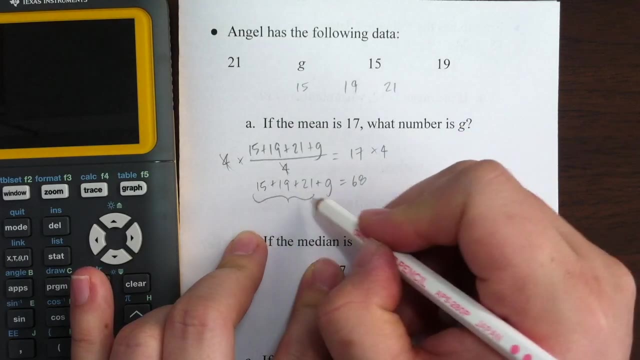 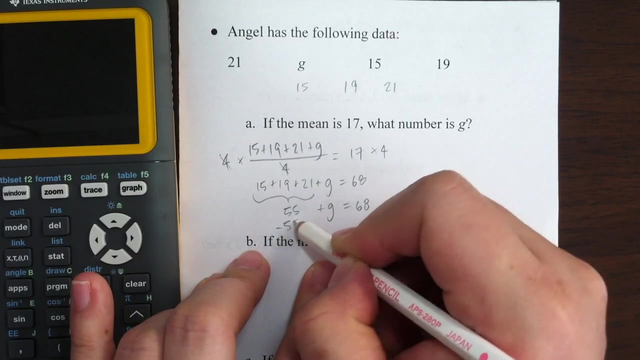 This is divided. so I multiply 4, divide 4 is 1.. 17 times 4 is 68.. I can add these numbers first, 15 plus 19.. 17 plus 21 gives me 55. I subtract 55 to eliminate. 55 minus 55 is 0. And here I have G. 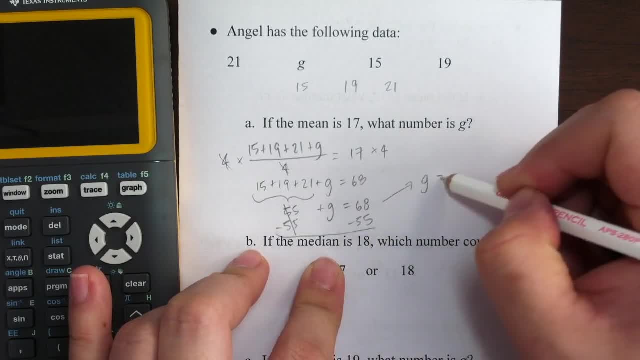 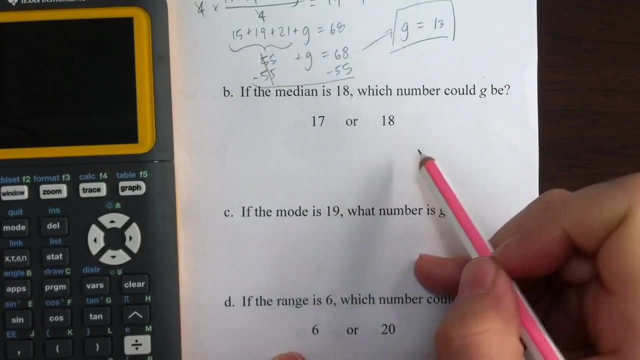 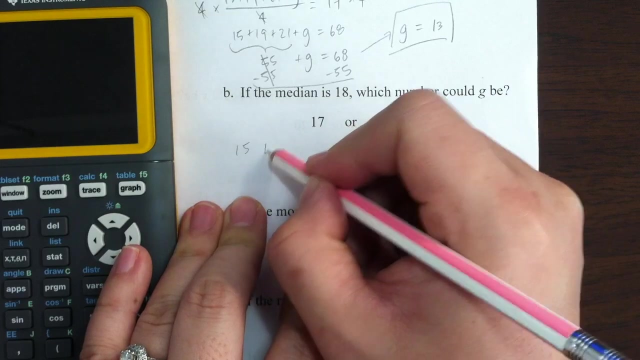 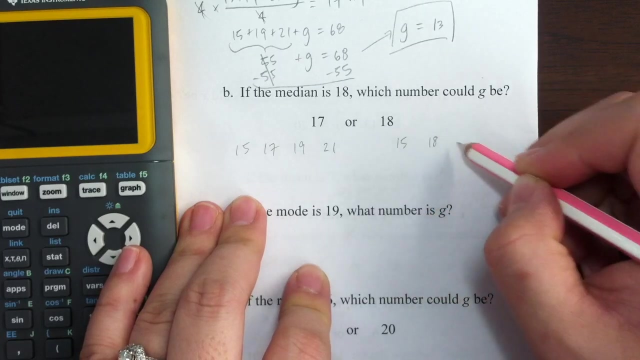 equals 68 minus 55.. G equals 13.. If the median is 18,, which number could G be? So if I have 15,, 17,, 19, and 21,, or 15,, 18,, 19, and 21,, let's find the median. I eliminate the outside numbers. 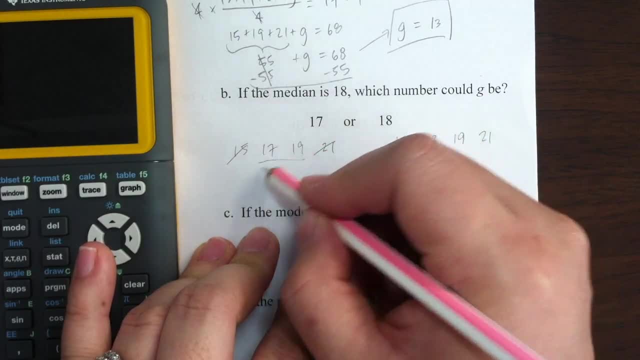 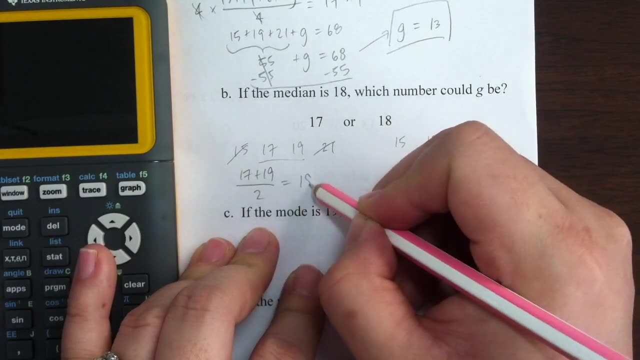 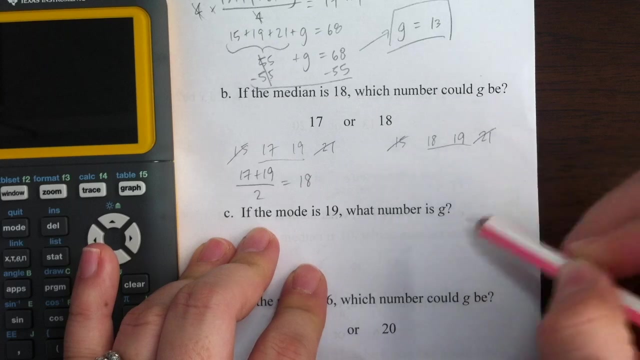 but then I have 2 in the middle. So I must take these 2, add them together and divide by 2.. This will give me 18.. Just to check, I'm going to try the other ones. Eliminate the outside numbers And I have 2 in the middle. So 18 plus 19, divide by 2, gives me 18.5.. 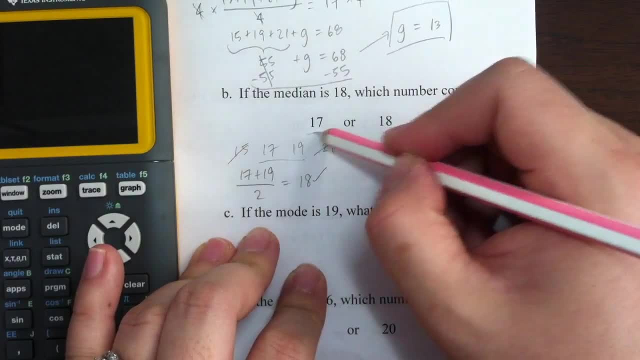 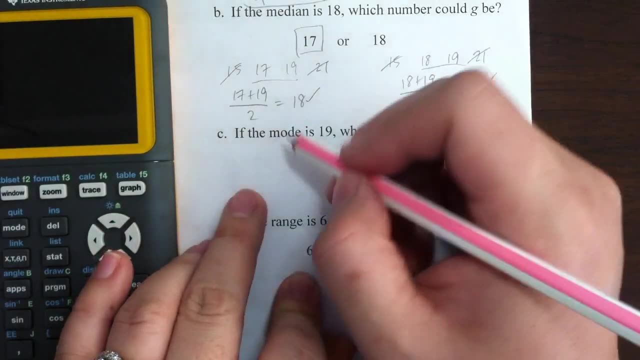 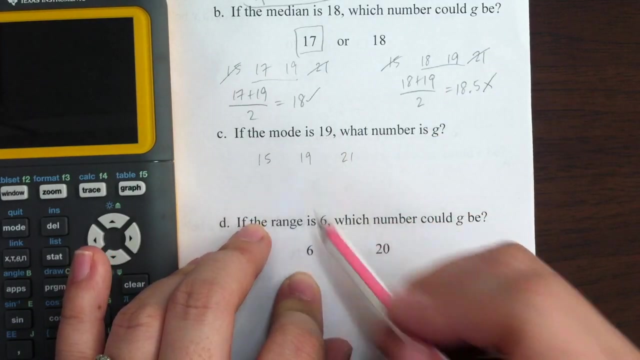 I want median 18,, not 18.5.. So my answer will be 17.. If the mode is 19,, what number is G? So I have 15,, 19, and 21.. I want mode to be 19.. I need to repeat 19.. 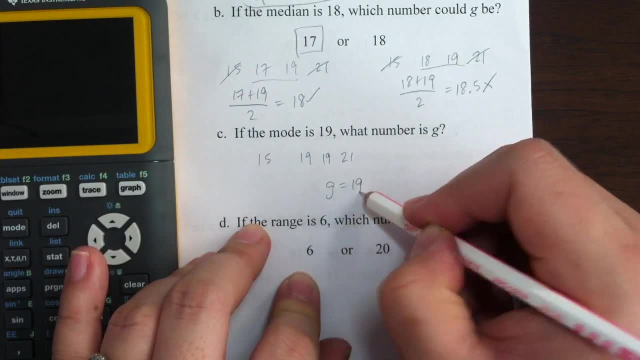 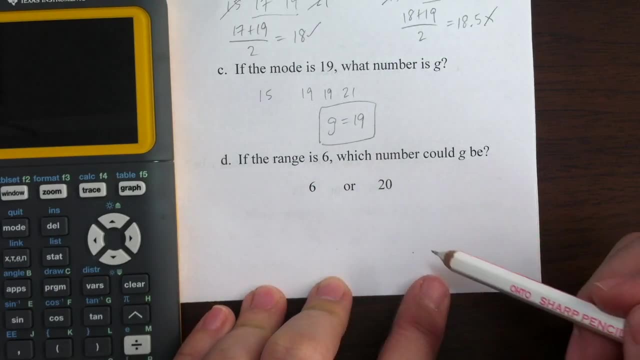 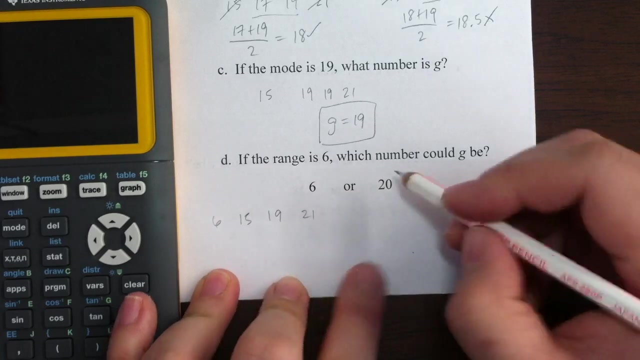 So I must have: G equals 19.. And finally, for this example, if the range is 6,, what number could G be? 15,, 19,, 21, and 6, or 15,, 19,, 21, and 20.. 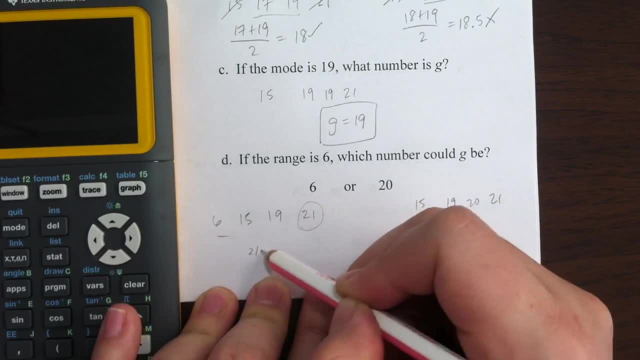 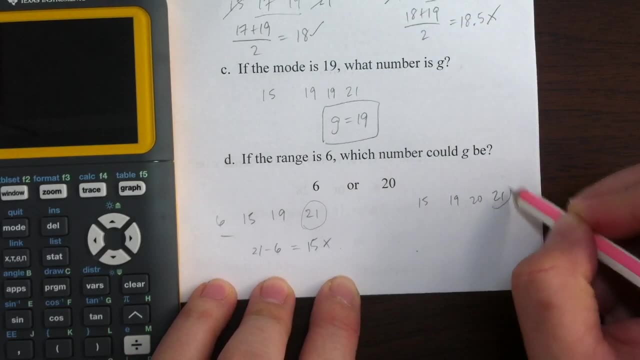 So remember, range is the largest number minus the smallest: 21 minus 6,, 15,, which is not what I want. Or 19,, 19,, 21, and 20.. 21 minus 15 equals 6,, which is what I want. 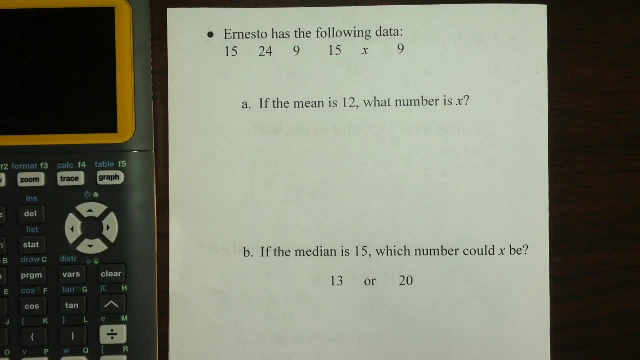 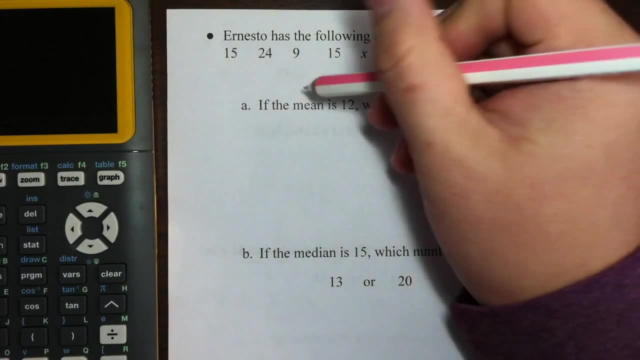 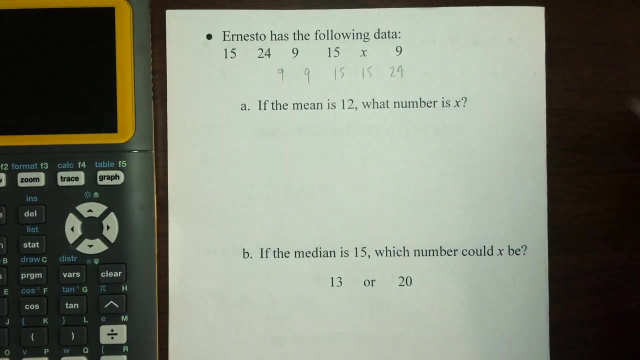 So my answer should be 20.. Ernesto has the following data: 15,, 24,, 9,, 15,, x and 9.. I'm going to write the numbers in order, leaving out the x. If the mean is 12,, what number is x? 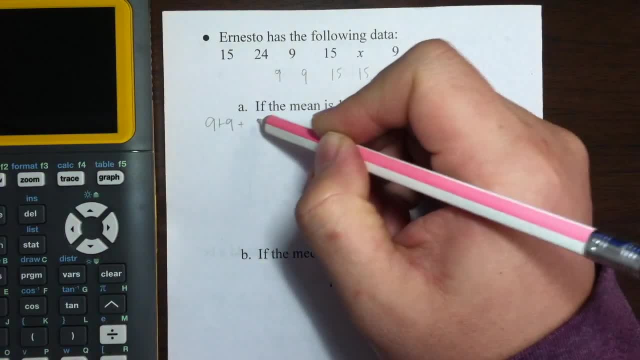 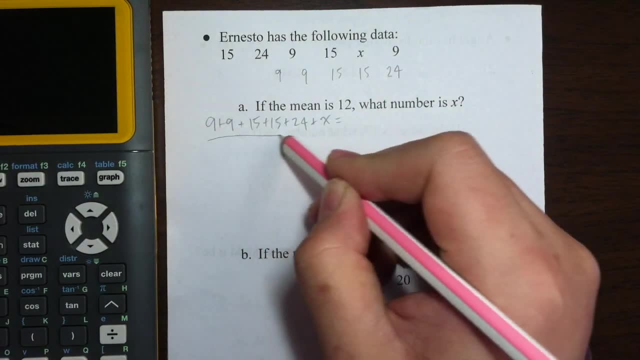 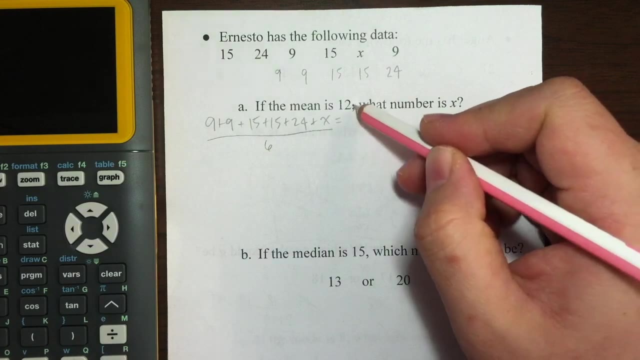 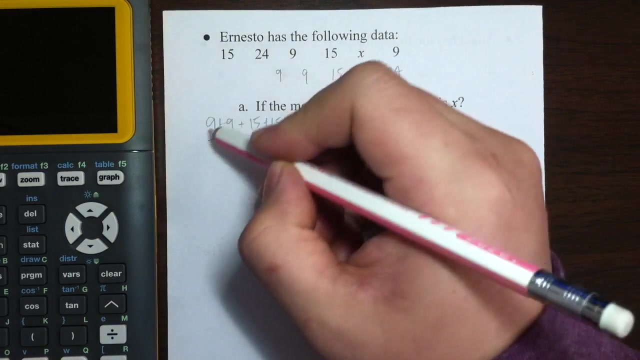 I'm going to add all the numbers together And when I divide, I need to divide 1, 2, 3, 4, 5, 6.. That will give me a mean of 12.. To eliminate the 6, because it's divided, I multiply. 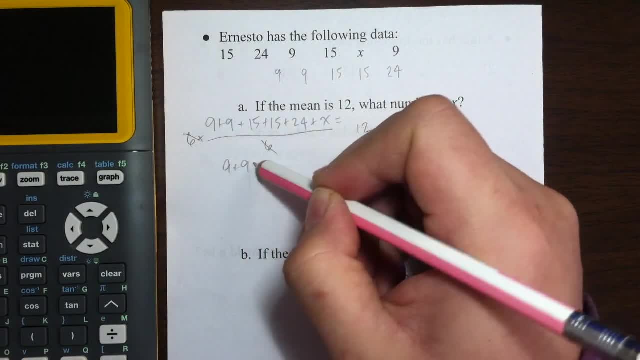 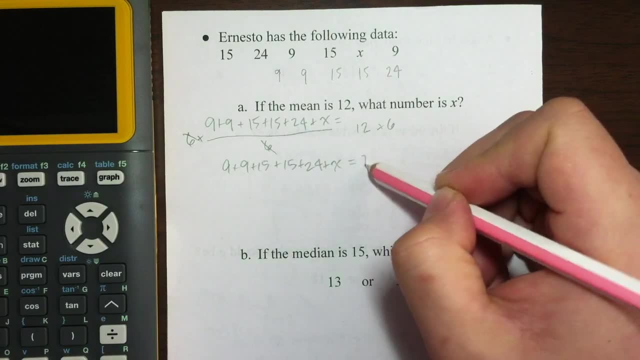 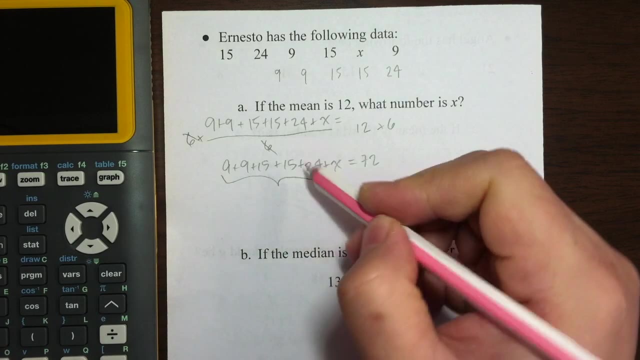 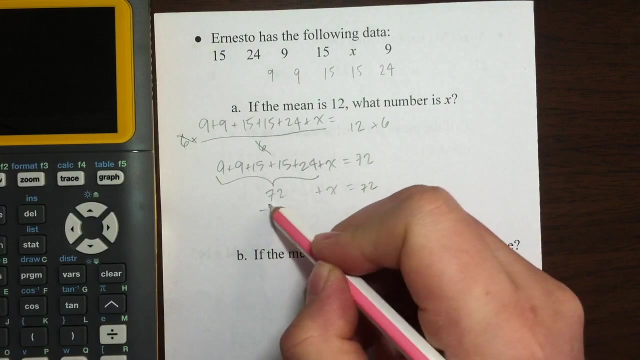 6 divides 6 gives me 1.. 12 times 6 is 72. And then I can simplify: 9 plus 9 plus 15 plus 15 plus 24.. That will give me 72. I need to eliminate the 72, so I change the sign to minus. 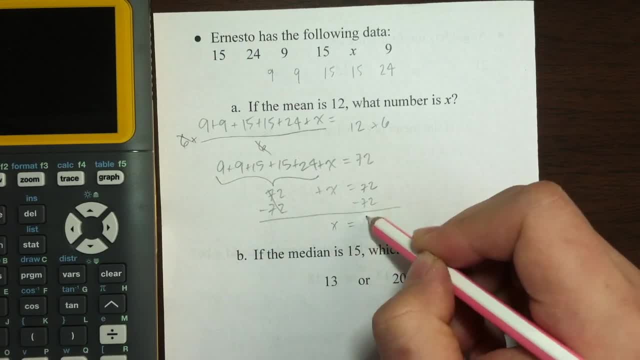 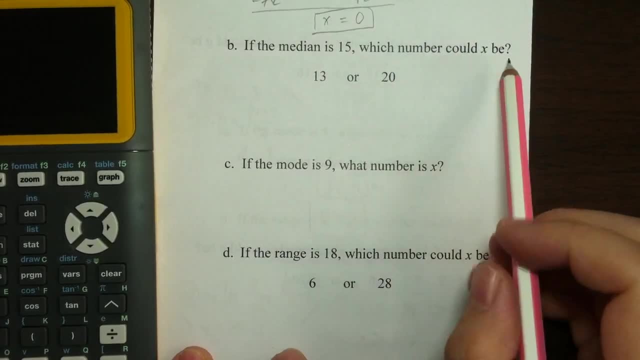 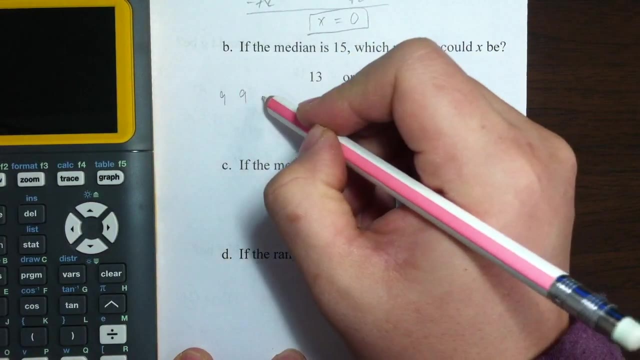 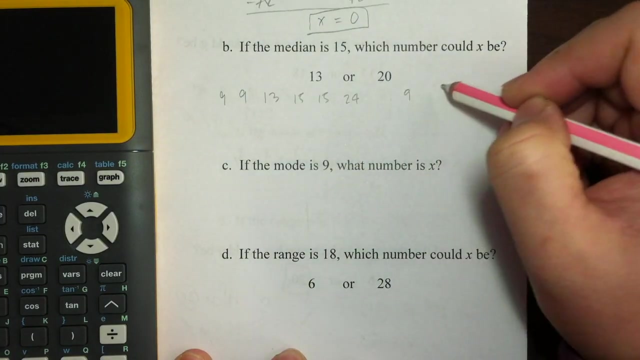 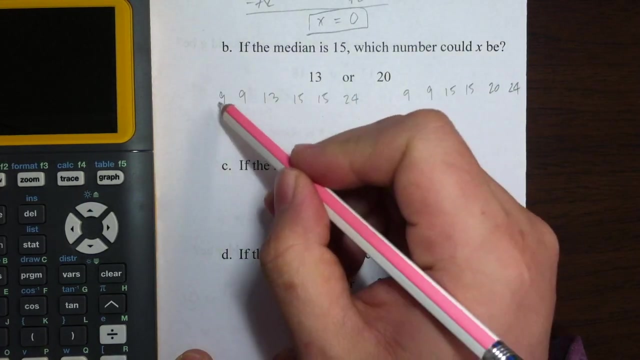 72 minus 72 is 0.. x equals 0.. If the median is 15,, what number could x be? 13 or 20.. So if I write the numbers with 13, or with 20,, let's look at the medians. 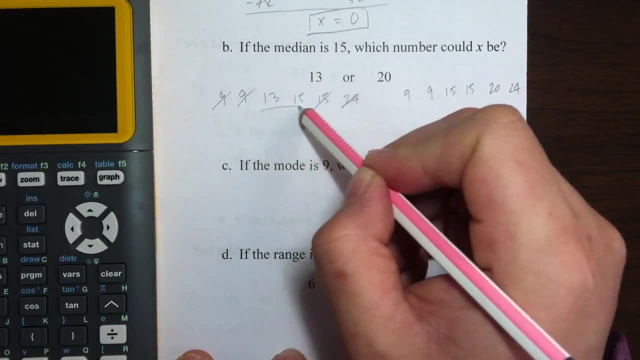 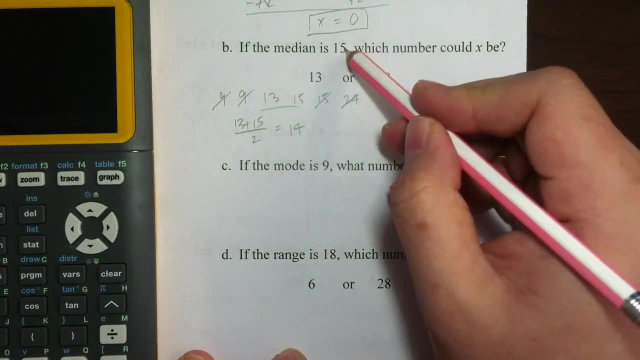 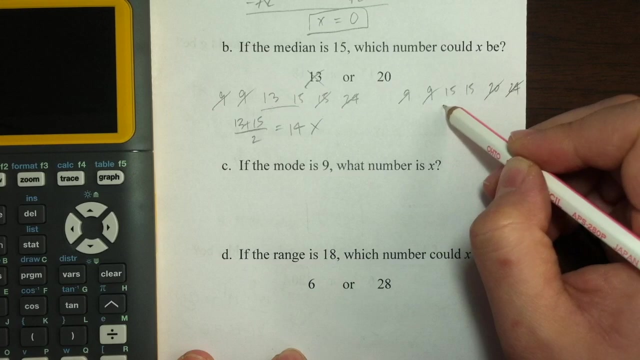 I eliminate the outside numbers- and I'm looking at the outside numbers- I'm left with 2.. So 13 plus 15 divide 2 gives me 14, which is not 15.. If I eliminate the outside numbers here, I have 15 in the middle. 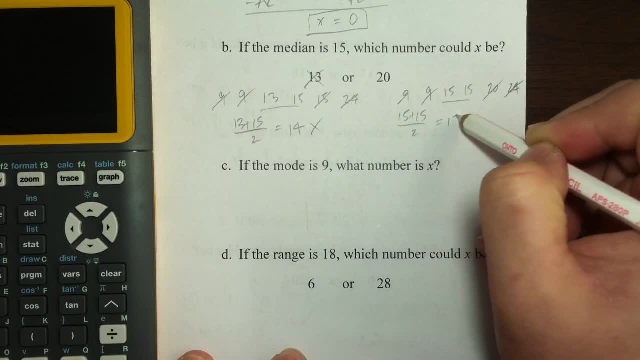 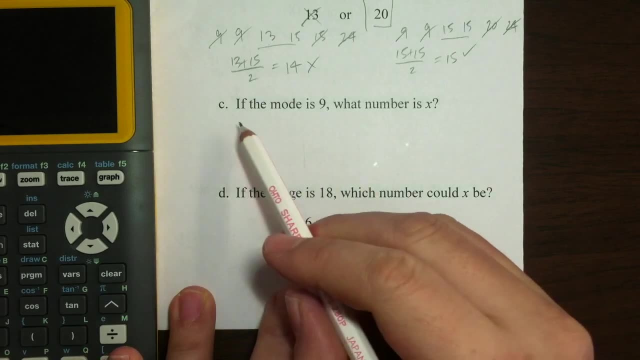 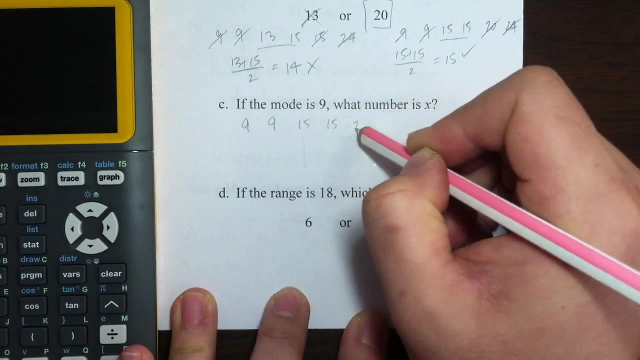 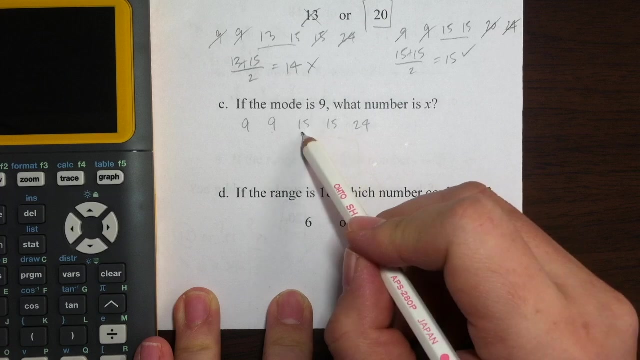 So that will give me 15.. If the mode is 9, what number is x? I want the mode to be 9, which means I need 9 to be repeated the most Here. I have 15 repeated and 9 repeated, but I want 9 the most. 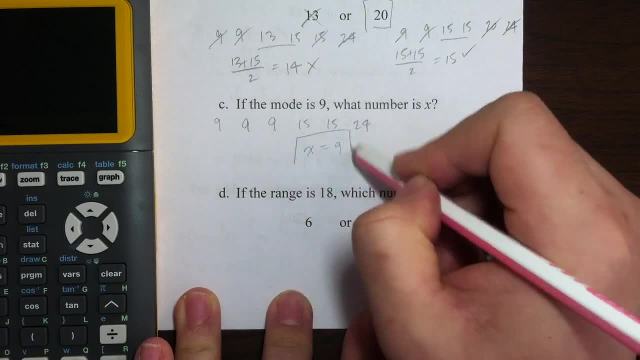 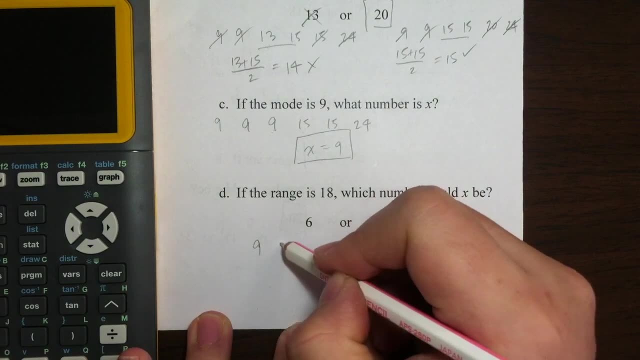 so I need to make another 9.. x equals 9.. If the range is 18, what number could x be If I write the numbers with 6,? what number could x be If I write the numbers with 6,? 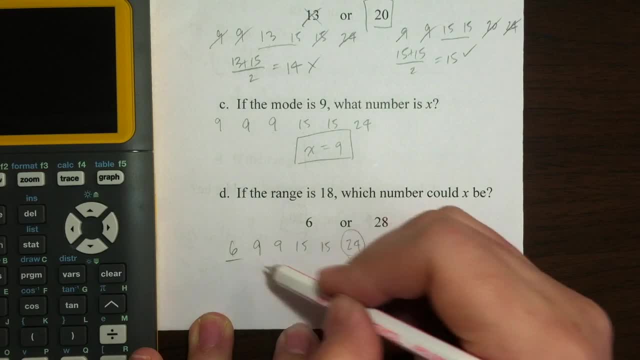 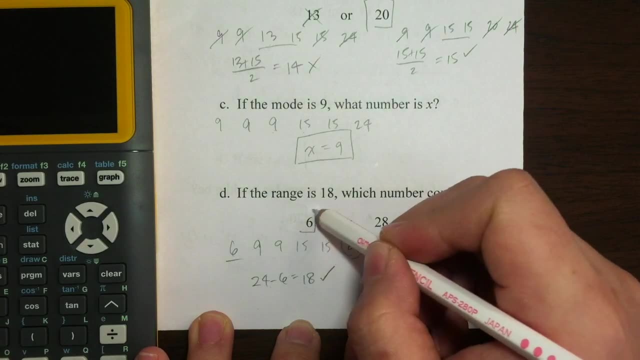 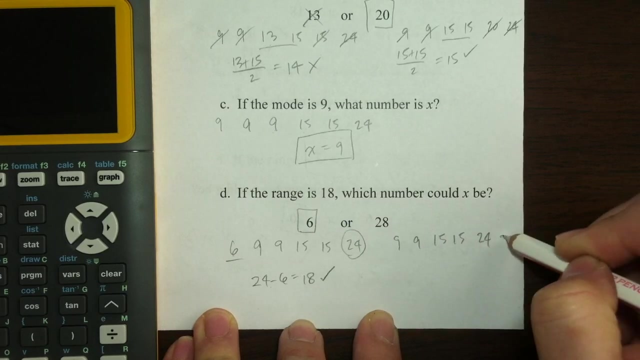 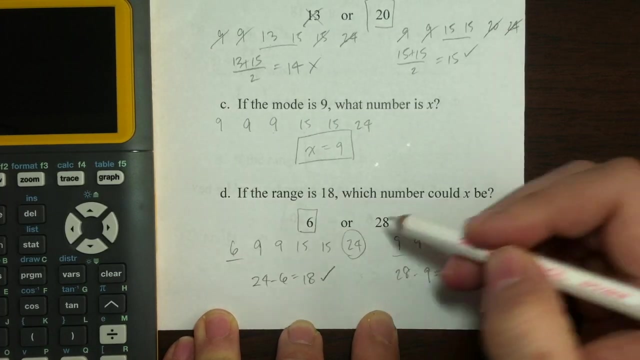 what number could x be? The answer is 6.. Then the range is 24 minus 6,, which is 18.. I'm going to check 28,. so I have 9.. 28 minus 9,, 19,, which is not what I want.